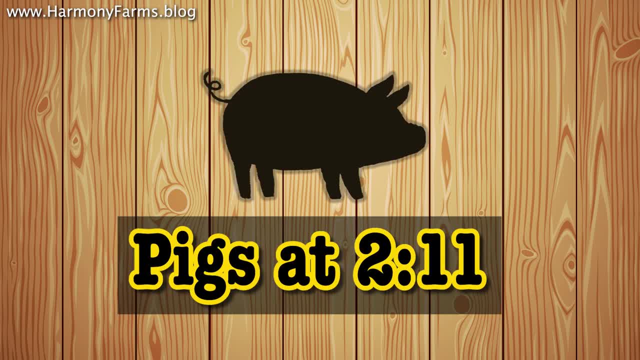 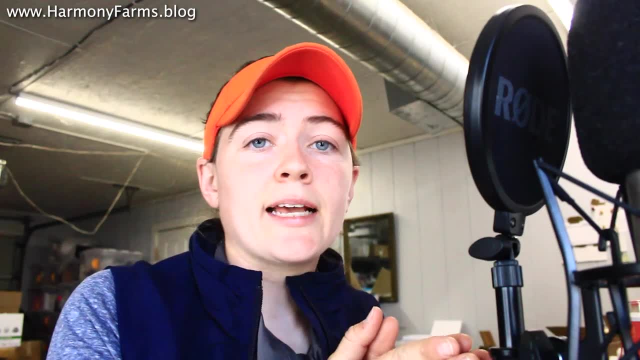 I'm going to list each species and how much food each animal provides, whether it's meat from a pig, beef, cow or lamb, or eggs from a laying hen. And number two, I'm going to talk about how long it takes to get that animal to. 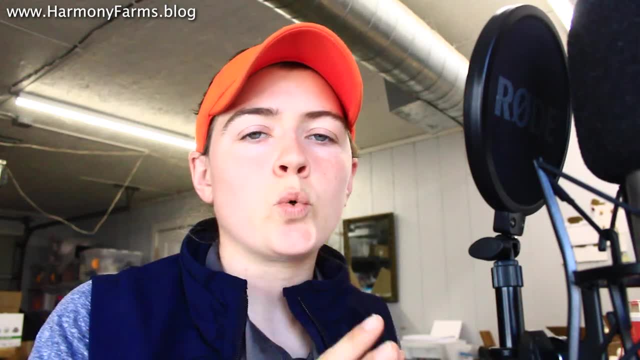 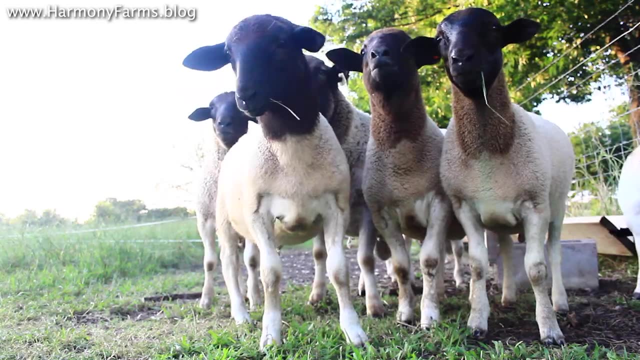 your plate Now, when you're growing an animal for food. there are two ways to really go about the growing process. Number one: you can buy a breeder pair and that pair has an offspring, and you can grow that offspring all the way up to butcher date. 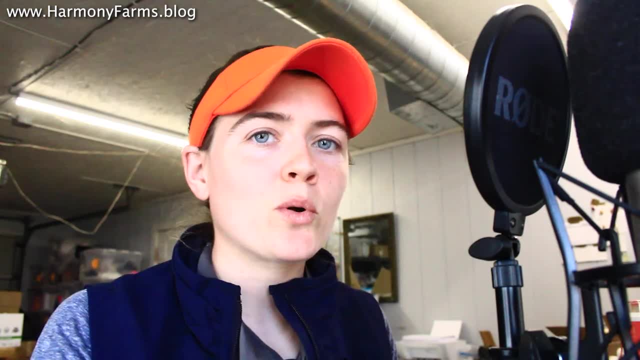 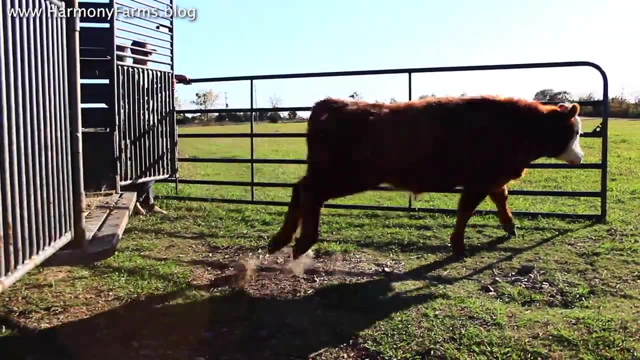 There's a second way that you can go about this and I'm going to be addressing this in a totally different video because I believe this is a great way for beginners to get in. But the second way is the stalker feeder route, And this is where you buy basically a half-grown animal from a ranch and finish out that animal and then butcher it. 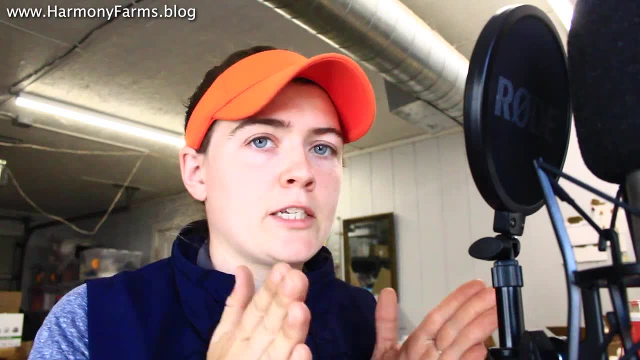 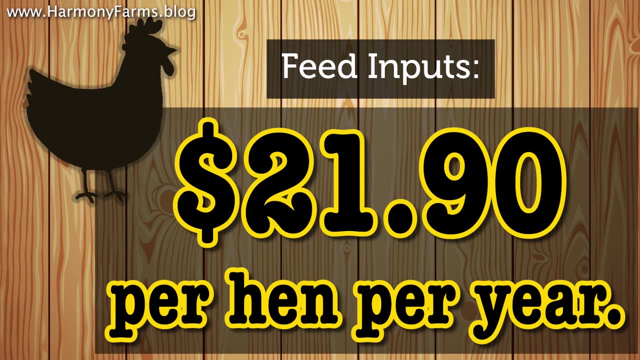 This video is going to assume that you are running a breeding program, meaning this animal is born on your farm and you grow it out to completion. I'm just going to start straight at the top with laying hens. In my previous video I stated that it takes about $21.90. 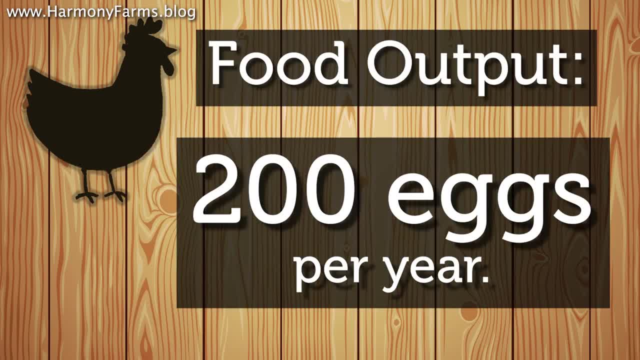 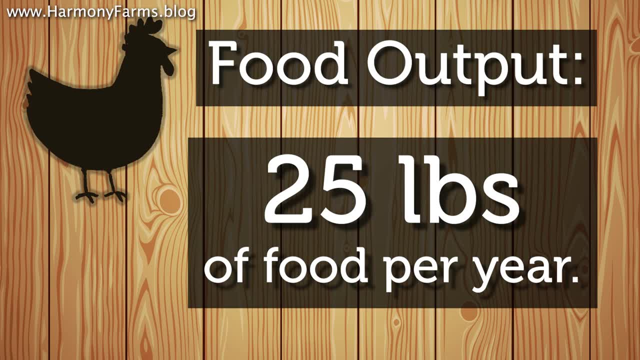 to sustain one laying hen for the course of a year, And over the course of a year you can expect about 150 to 200 eggs out of that laying hen, With each egg weighing about two ounces. you can expect about 18 to 25 pounds worth of edible products out of that laying hen. 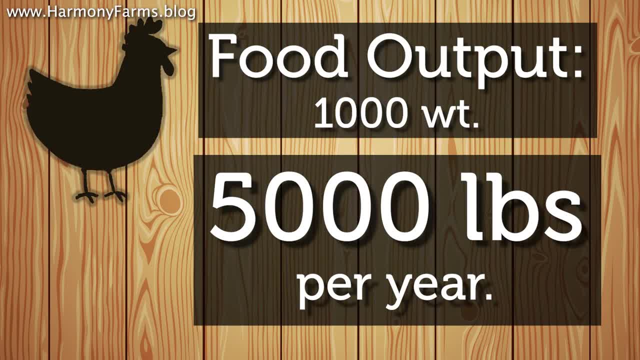 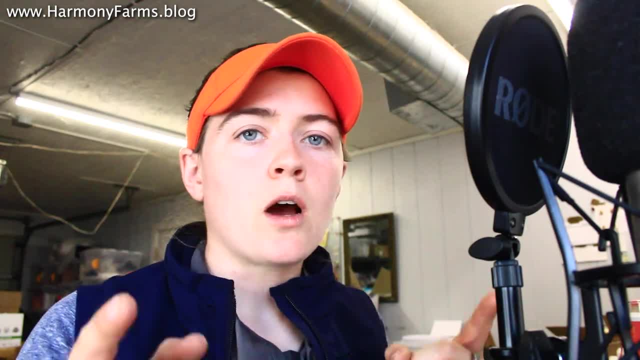 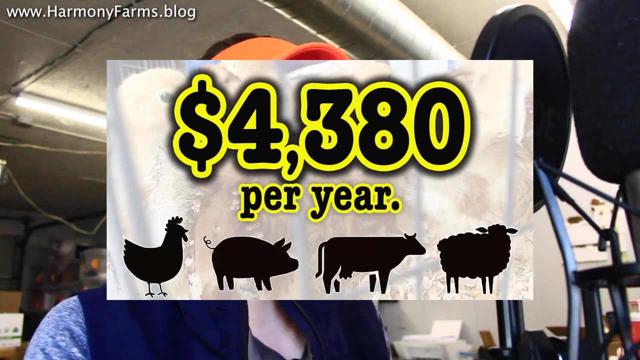 every year. This works out to roughly 5,000 pounds worth of edible product out of 1,000 weight of chickens per year, Which is really significant, and it's going to be the highest output on this list. If you guys go back to my previous video, you will see that laying hens require the highest amount of feed inputs. 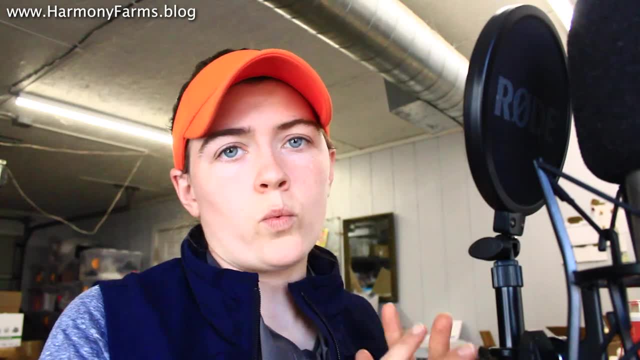 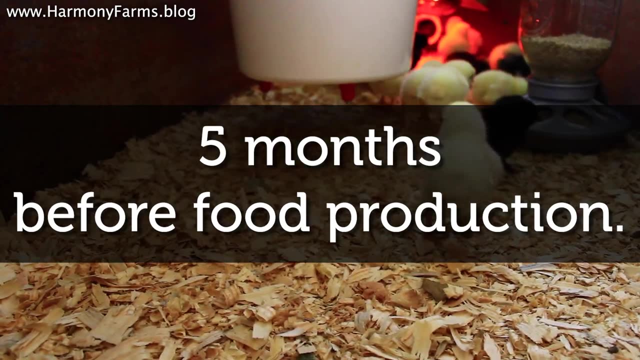 and they are the most expensive to keep per 1,000 weight with respect to all the animals on this list. But they really do carry their weight in the output category. When you get that baby chick in the mail it's going to take about five months before it lays you. 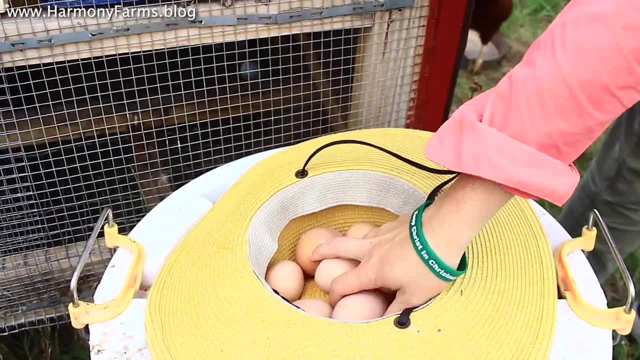 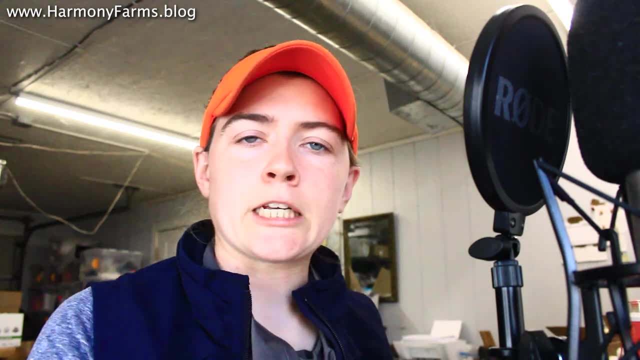 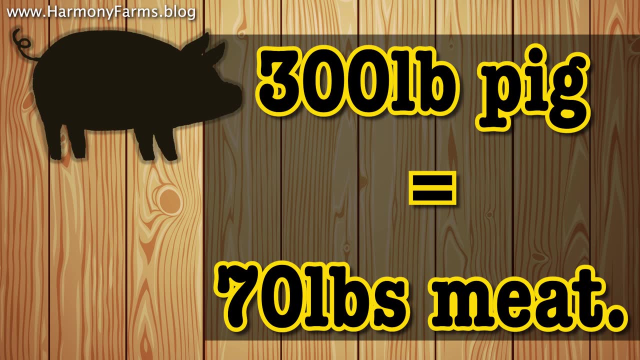 Now with a laying hen. this is a daily yield, except for over winter, when they pretty much produce no eggs, Unless you have a super chicken. If you do, comment down below and let us know how you raise a super chicken that lays 365 eggs per year. Moving on to pigs, A pig that finishes out at 300 pounds. 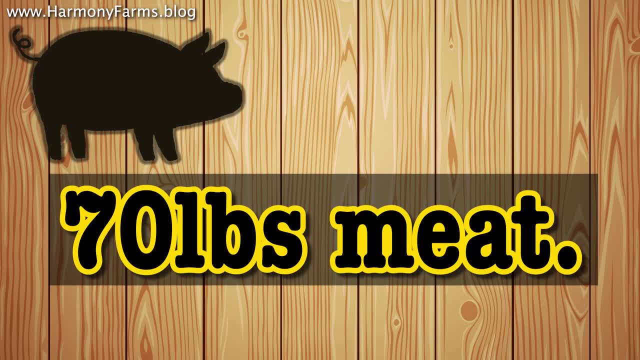 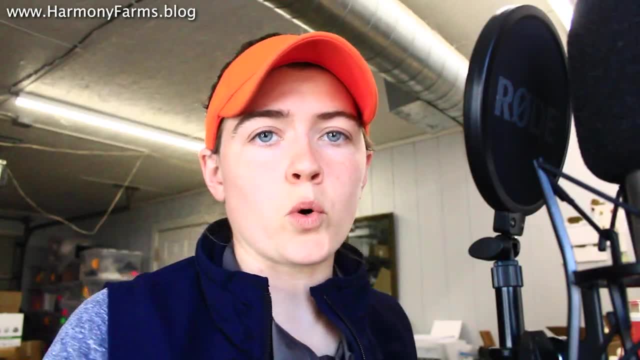 you can expect 70 pounds worth of packaged meat at the end of the day. You will be looking at about 231 pounds worth of meat on the table with 1,000 weight of pork Breeding to plate. you're looking at about 14 month time period for these pigs. 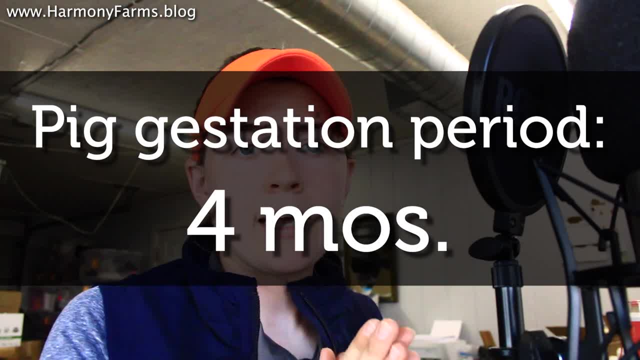 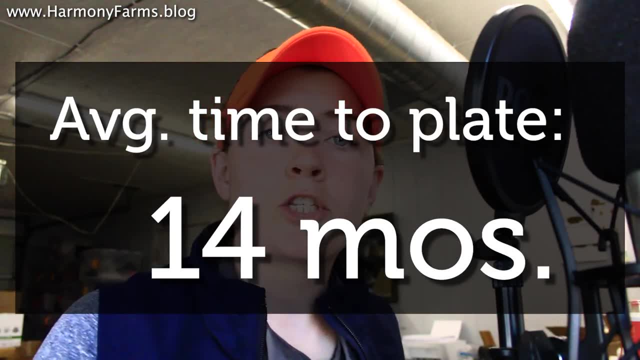 Pigs have a gestation period of three months, three weeks and three days. Once they're born, it takes around nine to twelve months to grow out a pig to 300 pounds, Meaning that at the end of 14 months you will be looking at a pork chop on your plate. 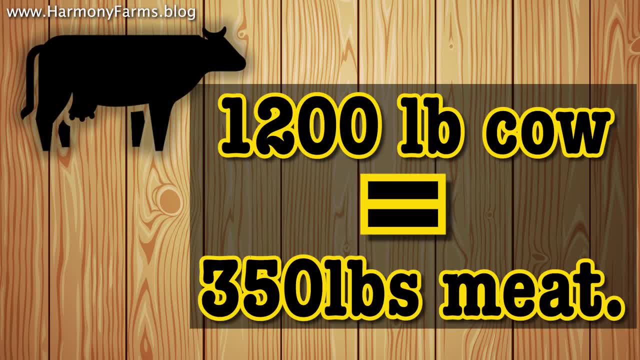 Number three on the list is a beef cow. A beef cow that finishes out at about 1,200 pounds. You can expect 350 to 400 pounds worth of finished meat In the freezer Once you are done. the beef cow is the longest from breeding to plate. 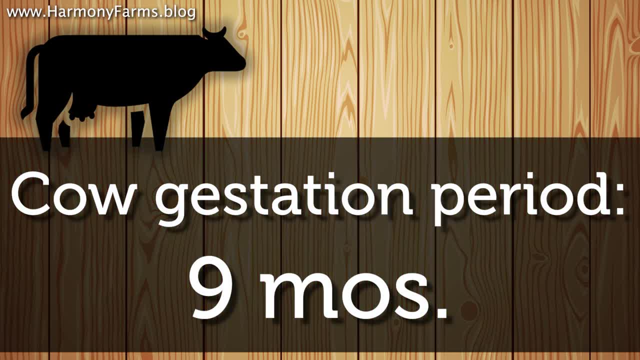 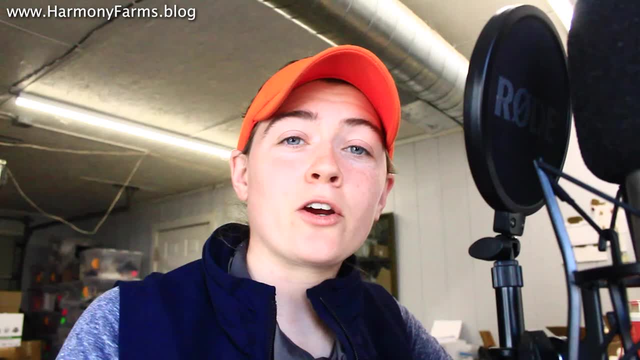 Once the animal is bred, it's a nine month gestation period. If you are finishing on grass, you are looking at 24 months to finish that animal. So you're looking at about a 33 month period from breeding to plate with the beef cow. 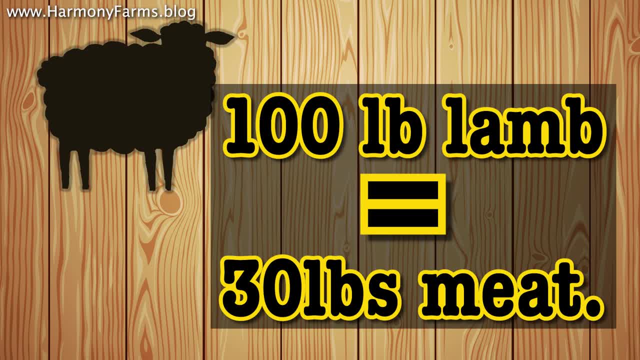 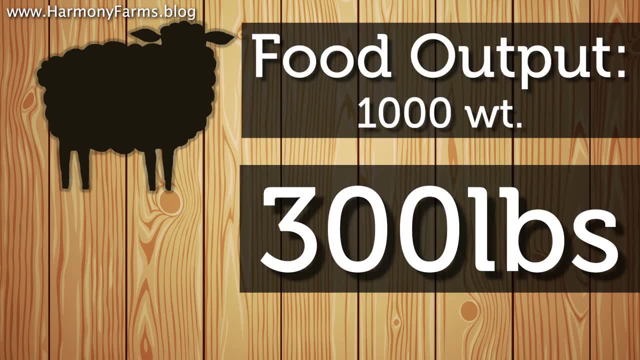 Number four on the list is sheep or lamb. The food output per animal on a well-finished, grass-fed lamb is around 30 pounds, And this is a lamb that finishes at 90 pounds. So you're looking at 30 to 100 pounds. 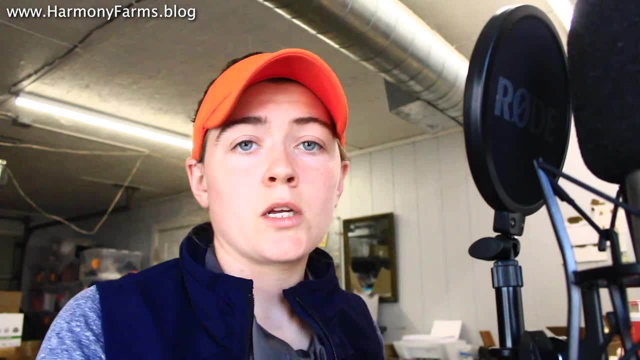 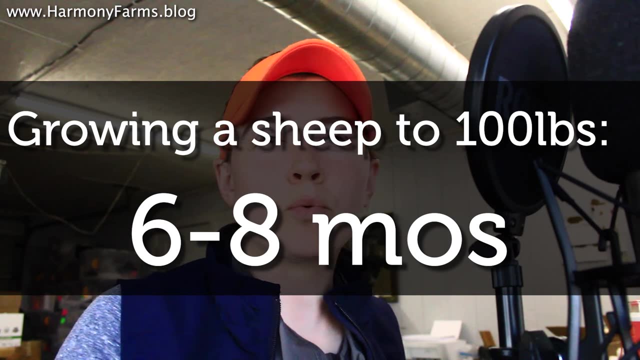 You have 10 100 pound lambs in 1,000 pounds. 10 times 30 is 300 pounds. Sheep gestation is five months And it takes about six to eight months to grow a Dorper lamb out to 100 pounds. 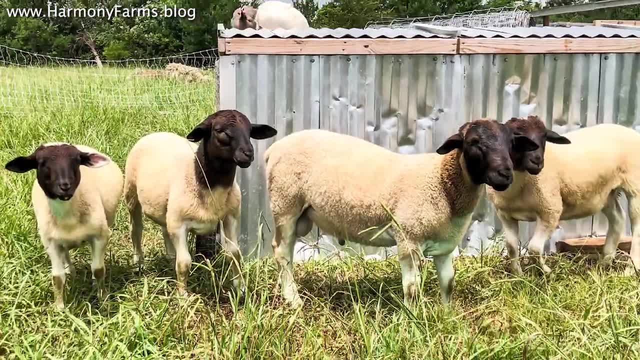 I want to make a quick note about finishing weights in general, No matter what the animal you're looking at And you want to really key in on the breed here And even the genetics coming off of the farm, Because these numbers that I am listing, these are good numbers. 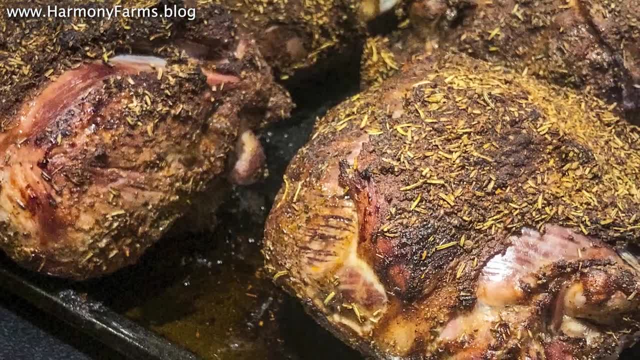 So when I say 30 pounds of meat off of a six to eight year old lamb, I'm talking about a six to eight year old lamb. I'm talking about a six to eight month finished lamb. I'm talking about the Dorper sheep. 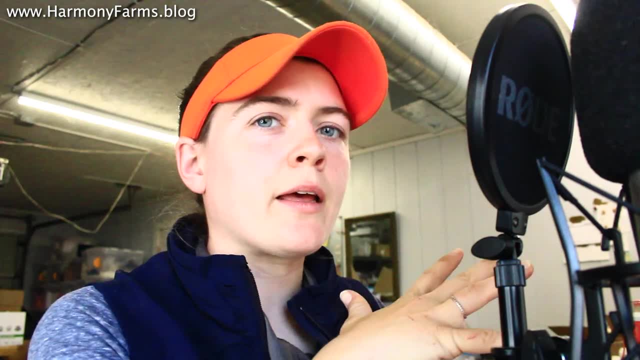 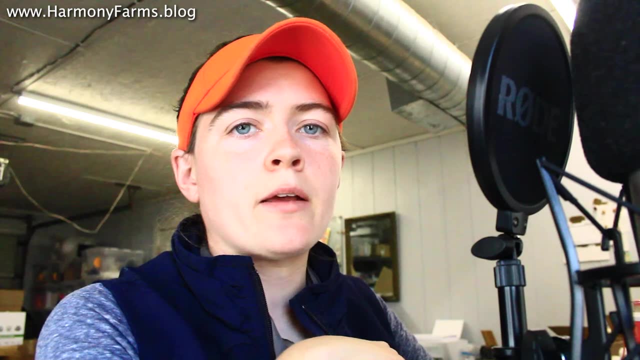 Now this is something I want to really ask you guys to comment below With respect to any lamb or sheep growers: How long does it take you to get your lamb to that good finished weight And what breed are you running When it comes to any animal- beef or lamb- finishing them out on grass? 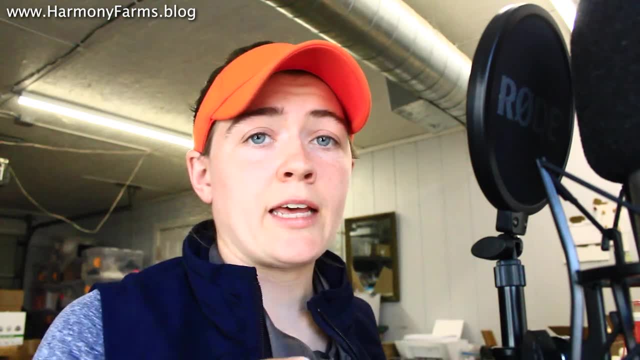 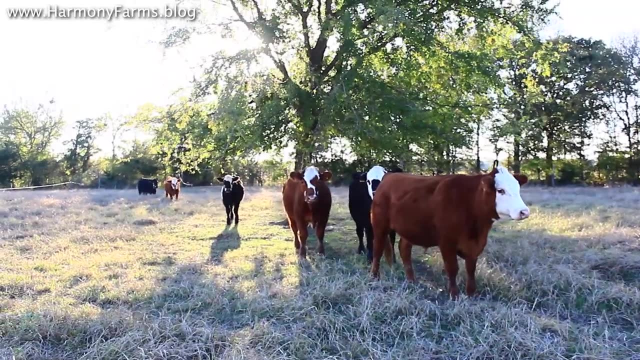 you really need to kind of key in on a specific genetic set, Find an animal that really is geared towards a grass-based system When you're in the context of finishing something out on pasture. In fact, I put together a whole article on that.